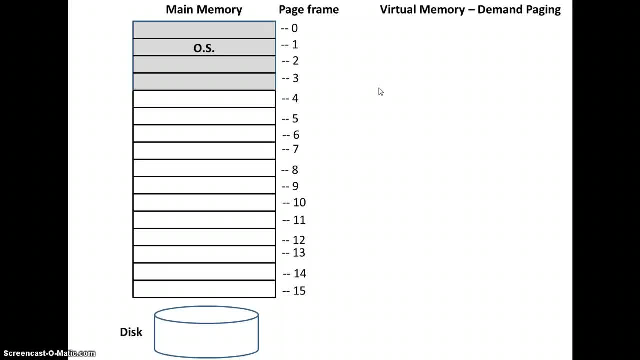 in time. here we are and that the only thing in memory is the operating system. And now we go to start a job. Well, since all of these pages are free, if we start a job, then it can use as many of the pages that that job requires. 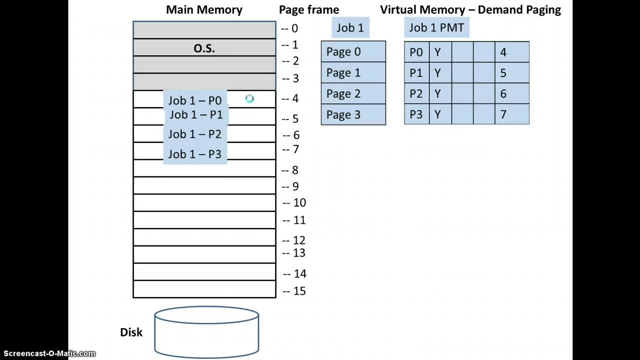 So let's say we have here this job one, and this job one requires four pages. Well, since pages four, five, six and seven were free, then we allocate those to this job one. So here our page map table is showing for job one, the page, the yes meaning that it's memory. 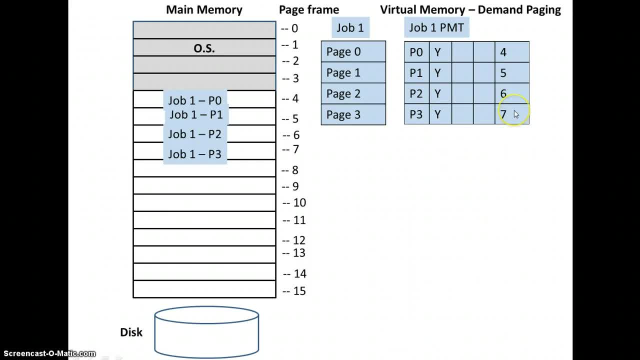 and then this last column is the actual frame that it represents. We'll have a different video where we take a look at these other ones here and that is whether it's been referenced and modified. What will happen is, as jobs start and take up more pages, then jobs end and some pages 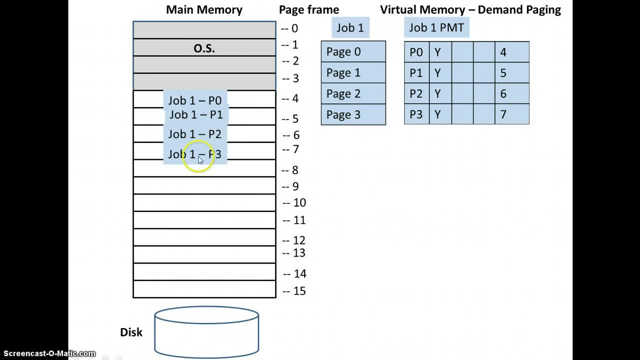 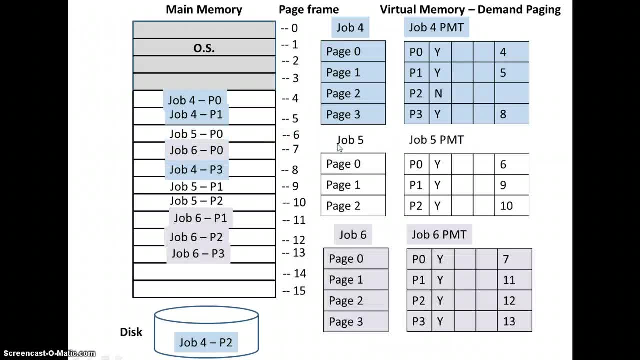 free up. the other thing that will happen is, if a page isn't referenced in a while, it will get removed from memory. So what I want to just show right here is: here's just a snapshot in time where there's three jobs that are running: Job four, job five and 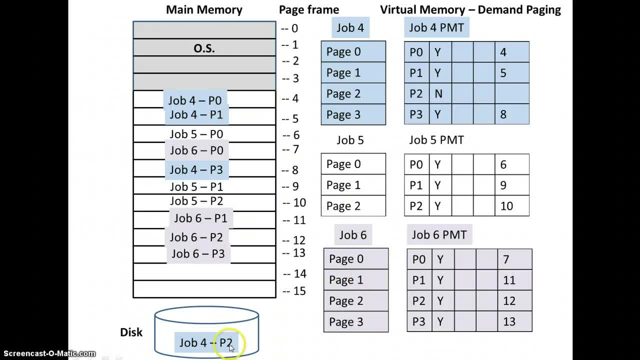 job six, And, as you can see, that For one of the jobs, job four- one of the pages that it has is actually on the disk as opposed to memory. But now this job four, as we see here, has pages four, five and 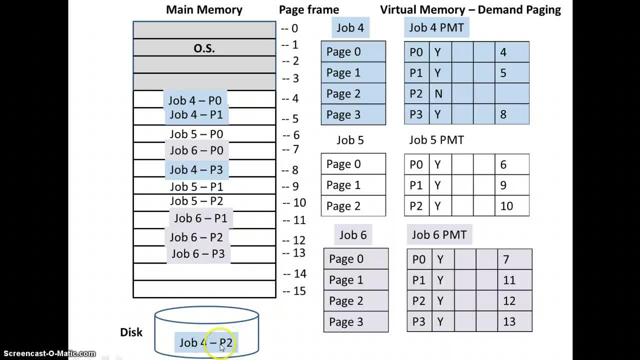 eight in memory, four, five and eight in memory. and then it has this page that's sitting here on the disk: Job five has pages six, nine and ten. Job six has seven, eight and ten. Job six has seven, eight and ten. 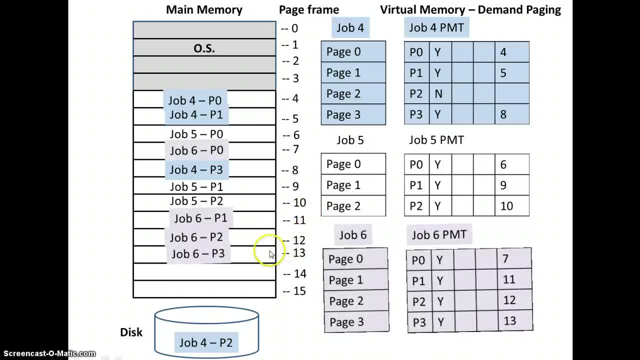 Job seven, eleven, twelve and thirteen, But suppose right now this job four is running and now it needs to reference the memory that is in this logical page two. Well, at the present moment this page is not in memory, so the end here. if we look at,